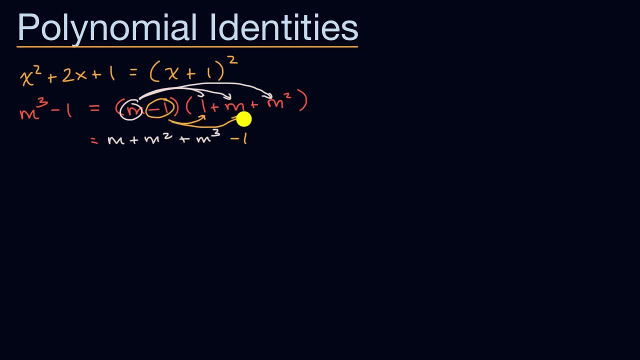 So negative one times one is negative one. Negative one times m is negative m And negative one times m squared is negative m And negative one times m is negative m squared. And now let's see if we can simplify this. We have an m and a negative m. 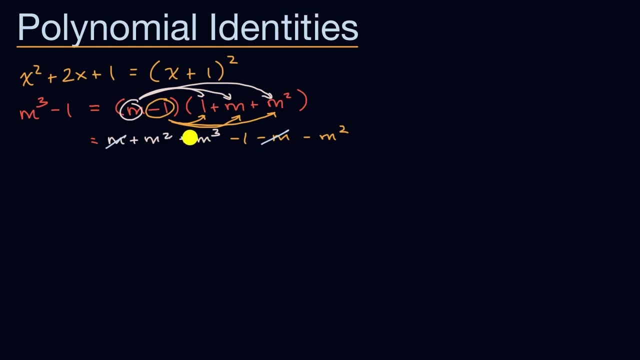 so those are going to cancel out. We have an m squared and a negative m squared, so those cancel out, And so we are going to be left with m to the third power minus one. Now, clearly, m to the third power minus one. 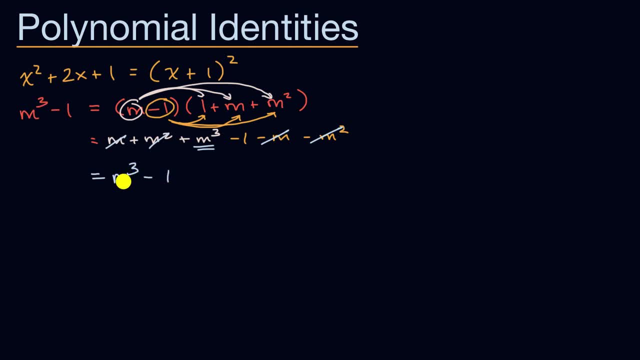 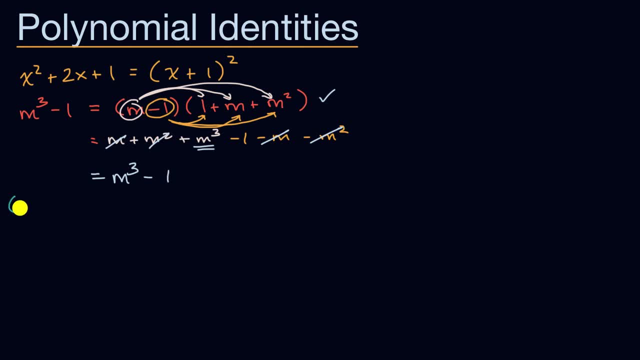 Let's say someone were to walk up to you on the street and said quick, n plus three, squared plus two n. Is that equal to eight? n plus 13? Is this a polynomial identity? Pause this video and see if you can figure that out. 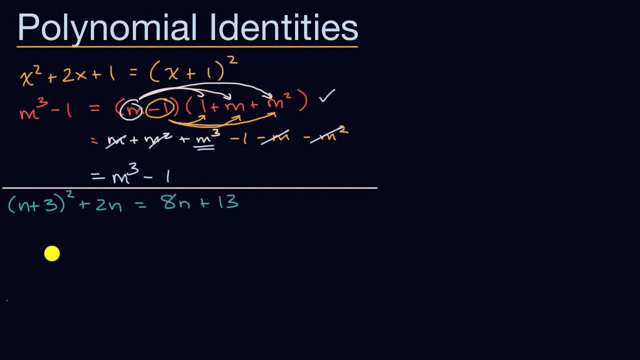 All, right, now we're gonna work on that together And I would do it the exact same way. I would try to simplify with a little bit of algebra, Maybe the easiest thing to do first, and you could do this in multiple ways. 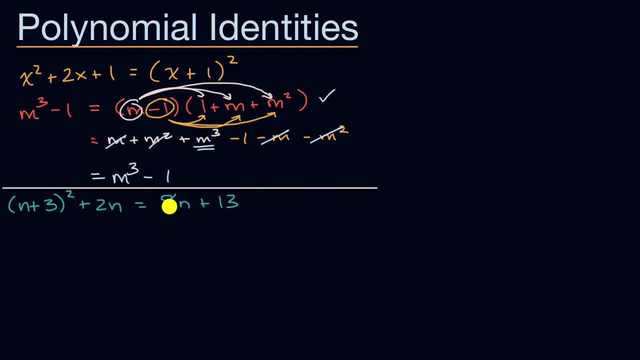 is, I have these n terms: two n's here, eight n's over here. Well, what if I were to get these two n's out of the left-hand side, So if I were to just subtract two n from both sides of this equation? 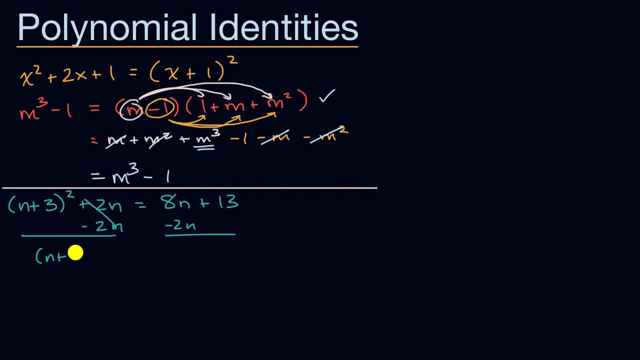 I am going to get, on the left-hand side, n plus three squared, And on the right-hand side, I am going to get six n eight, n minus two, n plus 13.. Now, what's n plus three squared? Well, that's going to be n squared. 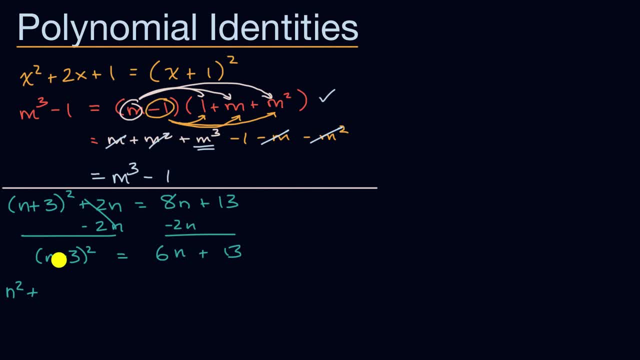 plus two times three times n. If what I just did does not seem familiar to you, I encourage you to look at the videos about squaring binomials. But this is going to be plus six n plus three squared, which is nine. 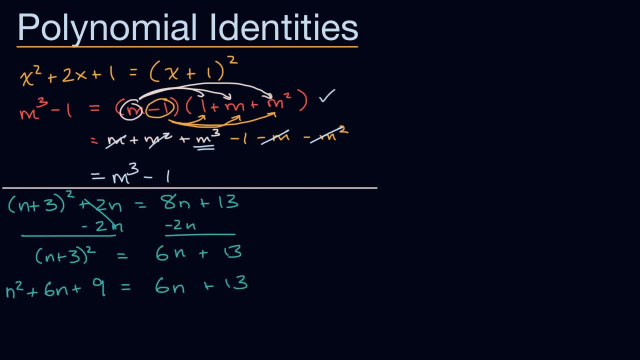 And is this going to be equal to six n plus 13? Well, already this is starting to look a little bit sketchy, but let's just keep going with the algebra. So let's see, If we subtract six n from both sides, what do you get?